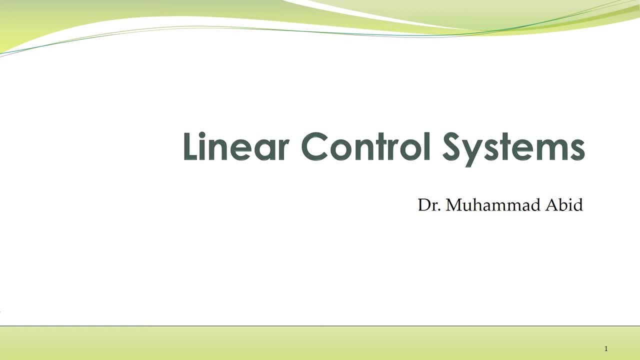 In today's lecture, we shall talk about mathematical modeling of physical processes. A mathematical model of a system describes the behavior of that system. There are different approaches to obtain a mathematical model. The approach that we shall follow in this course is based upon writing balance equations. 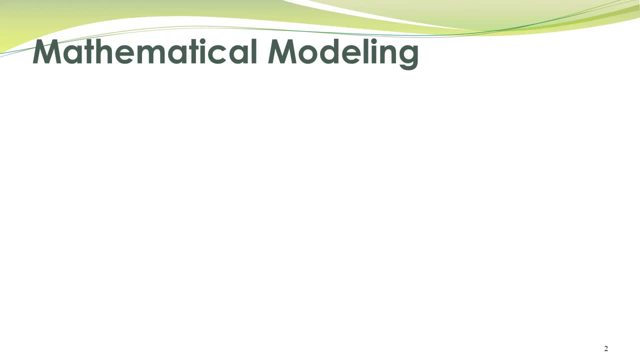 The systems that we shall talk about include electrical systems, electronic systems, mechanical systems, electromechanical systems and liquid levels. So let's first talk about electrical systems. Three basic elements in electrical networks are resistor, capacitor and inductor. 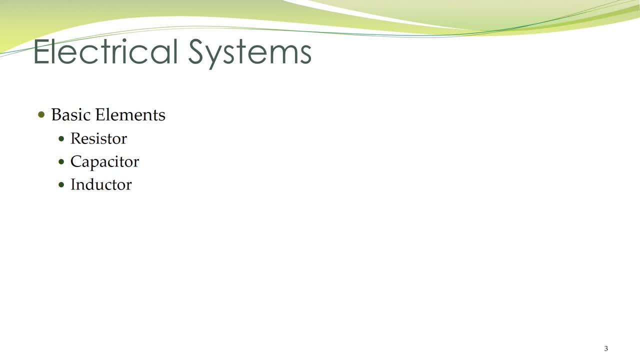 And the tools that are utilized to obtain a mathematical model for electrical networks are Kirchhoff's voltage law and Kirchhoff's current law, That is, KVL and KCL. You have taken at least two courses on circuit analysis, which describe analysis of electrical networks. 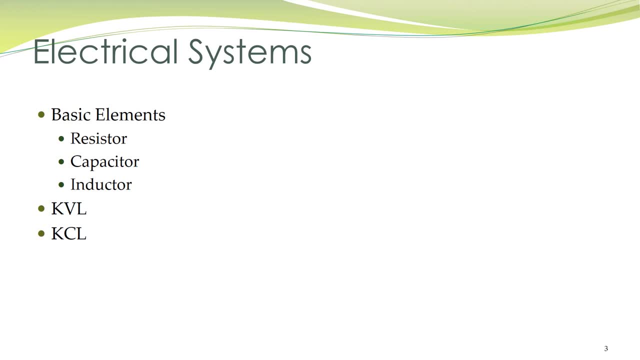 Therefore, we shall not spend too much time on this topic. We shall quickly go through two examples of electrical systems and shall describe their mathematical models. Consider, for example, a series RLC network as shown in the figure. A mathematical model can be obtained by applying Kirchhoff's voltage law. 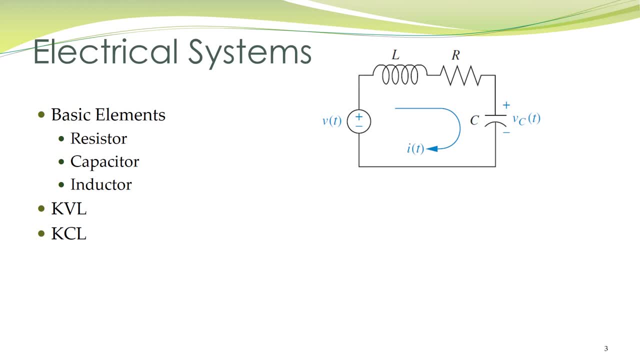 That is, sum of voltage drops is equal to sum of voltage rises, which is written in this equation: The first term is the voltage across inductor, The second term is voltage across resistor And the third term is voltage across capacitor, And sum of these voltages is equal to the applied voltage V. 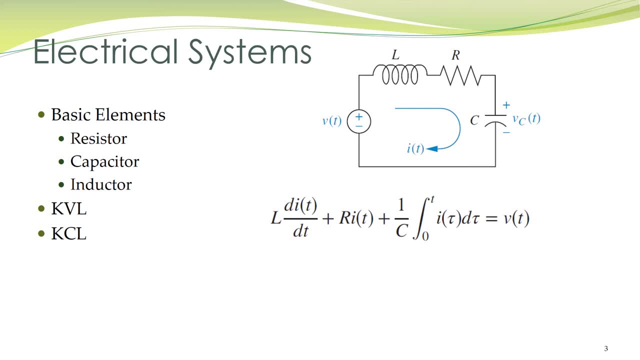 This is the first example. This is an integral differential equation by observing that current is nothing but derivative of charge, That is, I is equal to dq by dt. By this observation, the integral differential equation can be converted into a second order differential equation given by this expression: 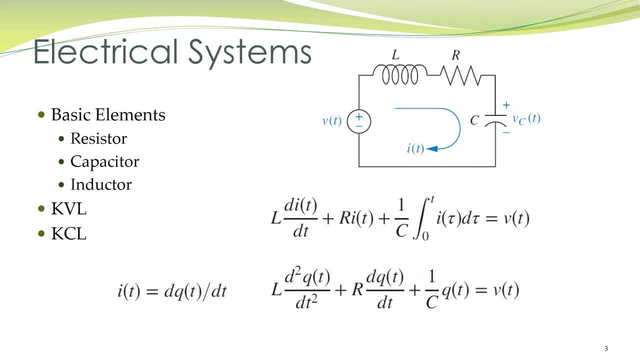 Therefore the term dI by dt is replaced by the second derivative of charge And the integral of current is charge. So third term is replaced by 1 over c q of t. The voltage across capacitor is given by Vc of t is equal to 1 by c q of t. 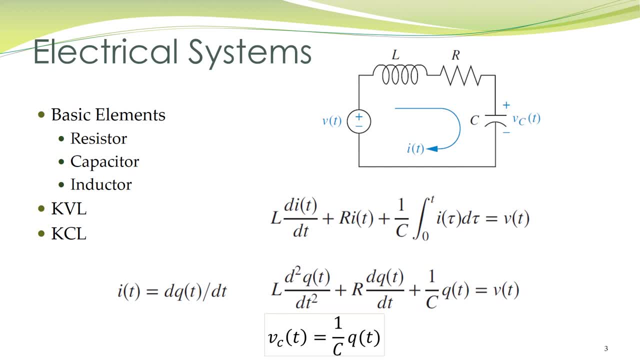 The last two equations describe the mathematical model for the electrical network. The system where there is a change involved are always modeled by differential equations. Such systems are called dynamic systems. So in this course we shall be mainly dealing with dynamic systems. 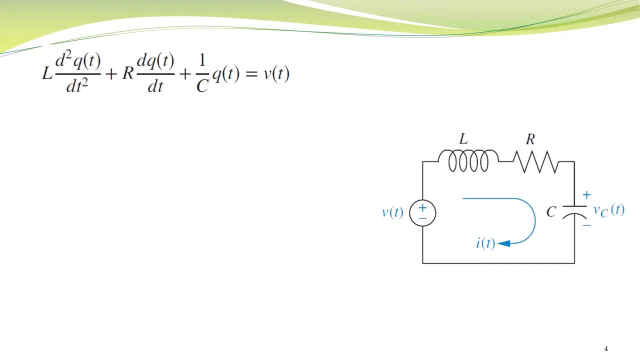 to find the solution of corresponding homogeneous equation, then finding the particular solution and then substituting the initial conditions to find the constants in the solution. 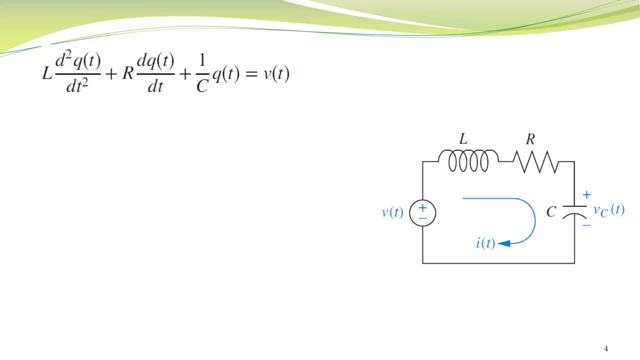 This procedure is quite cumbersome. An alternative approach is to utilize Laplace transform. You already remember that Laplace transform converts a differential equation into an algebraic equation, which greatly simplifies the things. Now let's take the Laplace transform of the differential equation. 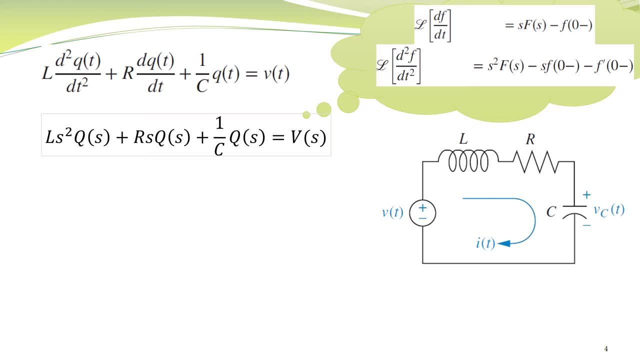 You remember that Laplace transform of derivative of a function, f of t, is equal to f of s minus f of zero, where f of zero is the initial condition. Let's take all initial conditions to be equal to zero. Thus the first equation, ie. 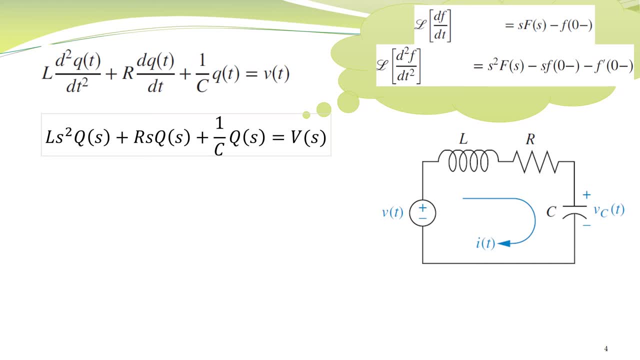 this slide, written in Laplace domain, is given by L s square Q of s plus R s. Q of s plus 1 over C, Q of s is equal to V of s. by taking Q of s common from the left hand side, we have the third equation on this slide, remembering from: 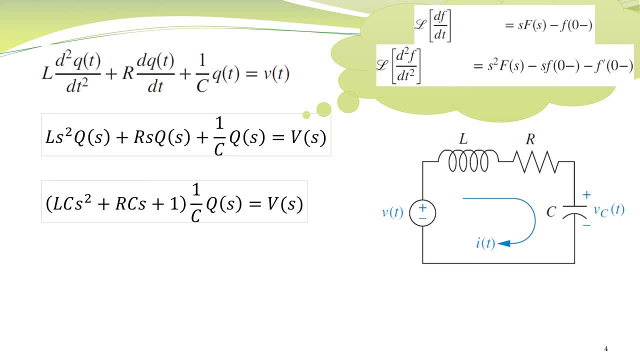 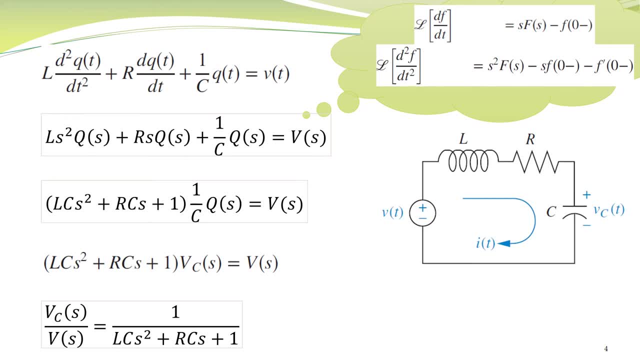 Q of s divided by V of s is equal to 1 over LCS square plus RCS plus one, which can be further rewritten as V. C of s over V of s is equal to 1 over LC divided by s square plus over LS, plus 1 over LC. this ratio, that is the ratio of laplace. 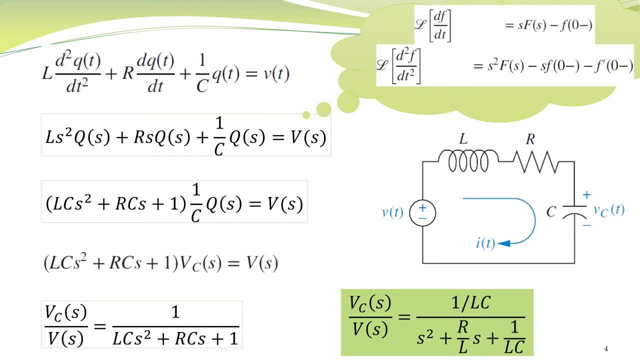 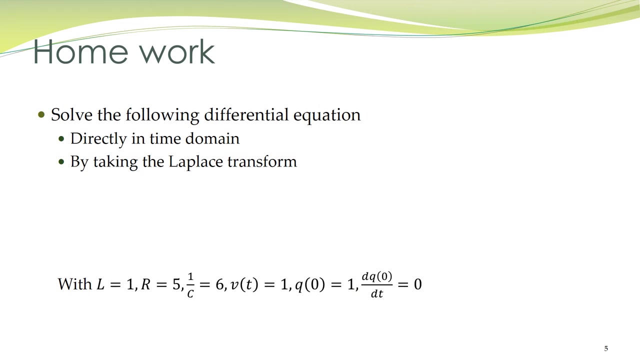 transform and Laplace transform of input with all initial conditions taken, equal to 0 is called transfer function of a system. Like differential equation, this transfer function also completely describes the system. Just to refresh your knowledge about differential equations and Laplace transform, I have a homework for you. You have not to submit it, but please do it. 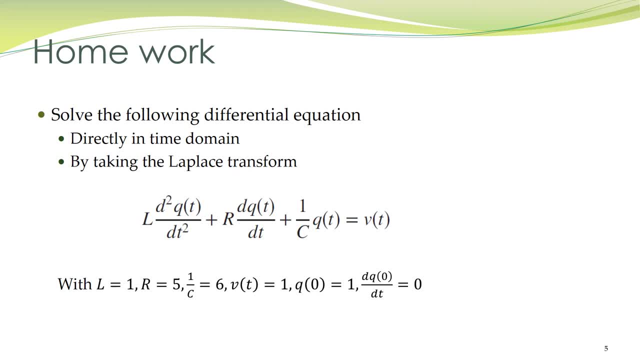 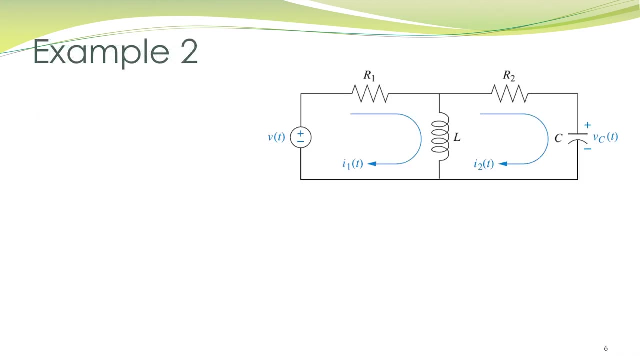 Solve the differential equation first directly in time domain and then by taking the Laplace transform of this differential equation. Now let's second. let's take the second example. We have an electrical network network over here with two loops. you already remember the procedure, the 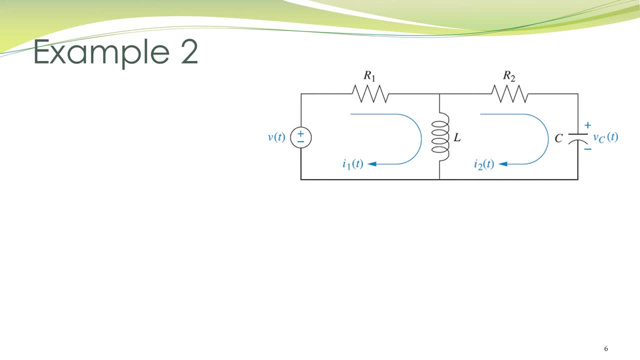 approach you are more convenient with is to rewrite the variables in Laplace domain, then apply KVL to obtain two equations. you are quite expert in analyzing electrical systems so I need not to explain this. I just write these equations over here. the first term in the first equation is the voltage drop. 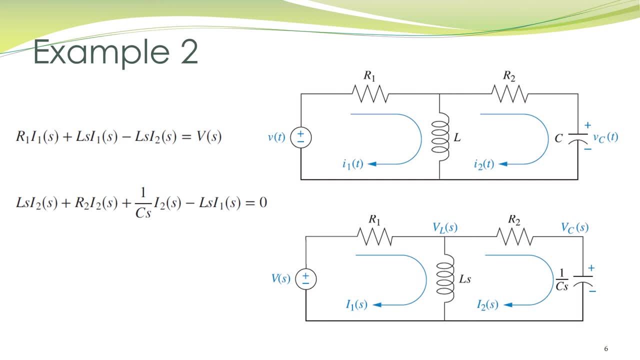 across the resistor. the second term, second and third term, or voltage drops across the inductor and the right-hand side of first equation is the Laplace transform of applied voltage. similarly, in the second equation, the second term is the voltage drop across resistor. the third term is voltage drop across the capacitor. first, 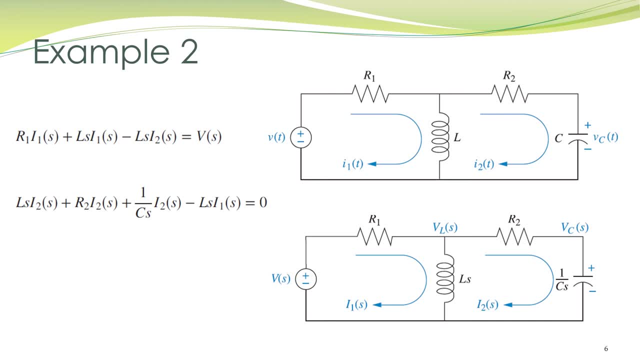 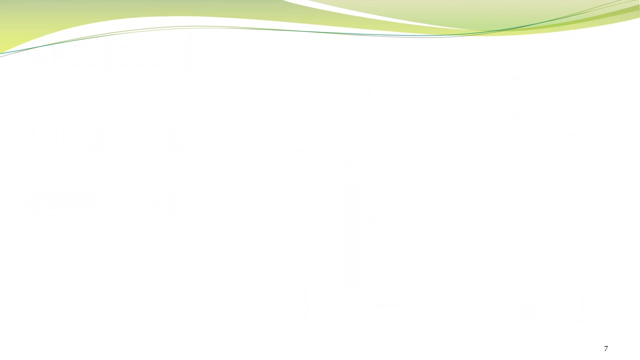 and fourth terms constitute voltage drop across inductor. the right hand side is zero because no external voltage is applied. so we have applied kvl to obtain a mathematical model for this electrical network. there is a shortcut which can be applied to describe, to obtain mathematical model in rather more conveniently. the two equations on the larts last slide are written: 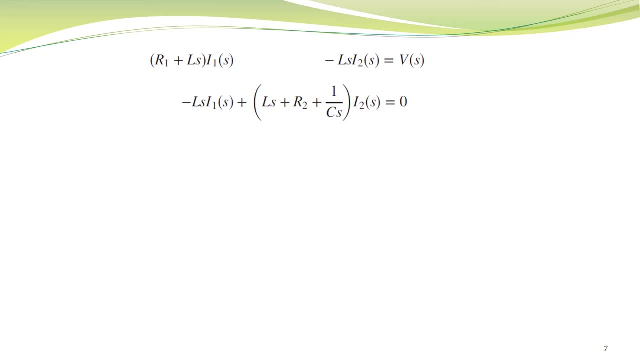 over here. if we look at these equations, we absorbed that in the first equation I 1 is being multiplied by sum of impedances in loop 1 and I2 is multiplied by a negative sign and sum of impedances common between loop 1 and loop 2.. The right hand side of equation is sum of applied voltages. Similarly, in equation 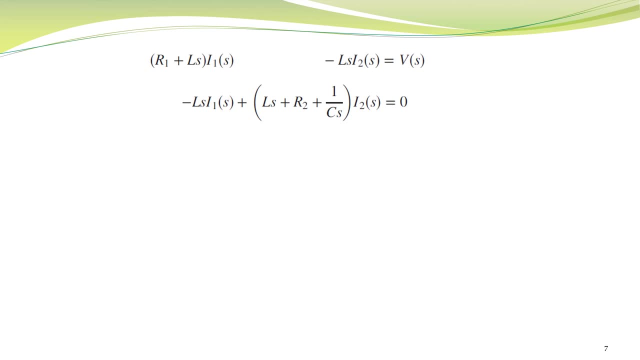 2, I1 of S is multiplied by a negative sign, and sum of impedances common between loop 1 and loop 2.. I2 is multiplied by sum of impedances in loop 2.. This observation is described below in words. that is, I1 of S multiplied by sum of impedances around mesh 1 minus I2 multiplied. 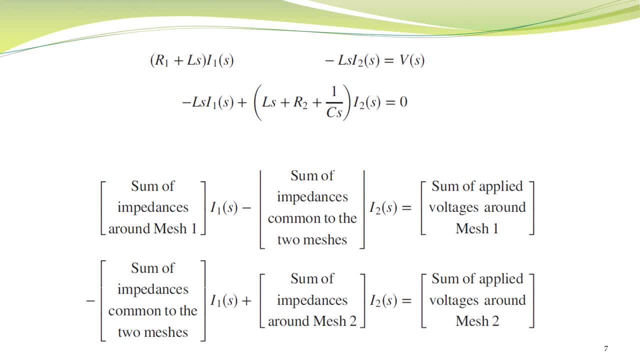 by sum of impedances common to the two meshes, and this is equal to sum of applied voltages around mesh 1.. Likewise, in the second equation, I1 of S multiplied by sum of impedances common to the two meshes with negative sign, plus I2 of S multiplied by sum of impedances around. 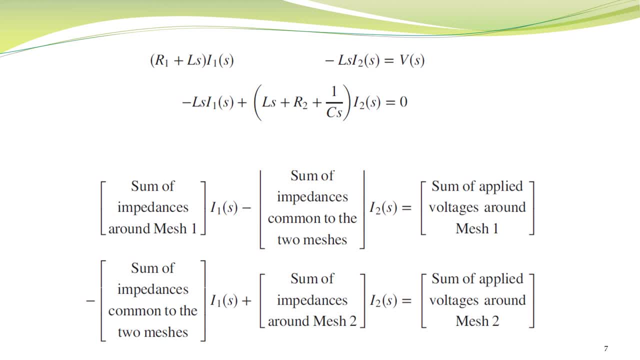 mesh 2.. This is equal to sum of applied voltages around mesh 2.. Thus we can get rid of even applying KVL. We can quickly write the equations describing the electrical, electrical, electrical network by using this shortcut. However, remember one important thing: This shortcut is applicable. 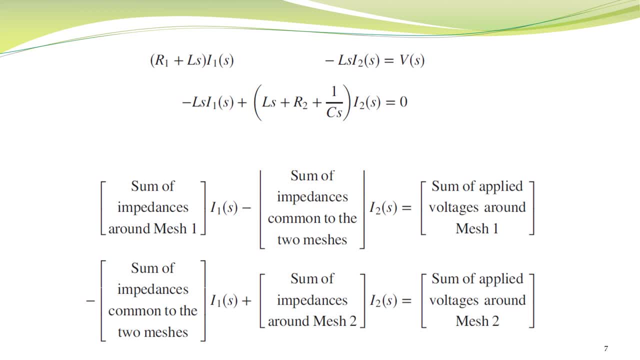 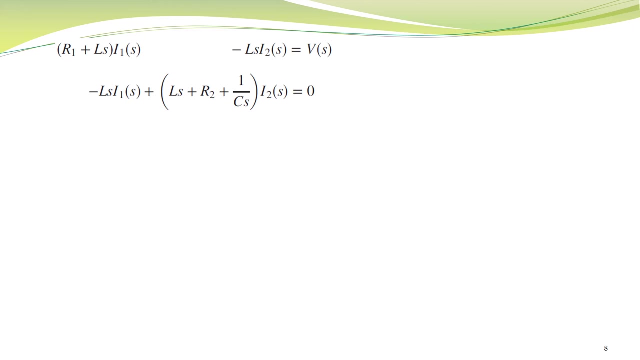 only if directions of current are as shown in the figure on previous slide. Otherwise, we have to make some changes in the signs of some terms in this equation. We have to make some changes in the signs of some terms in this equation. Again, we have the same two equations And now let's suppose that we are interested. 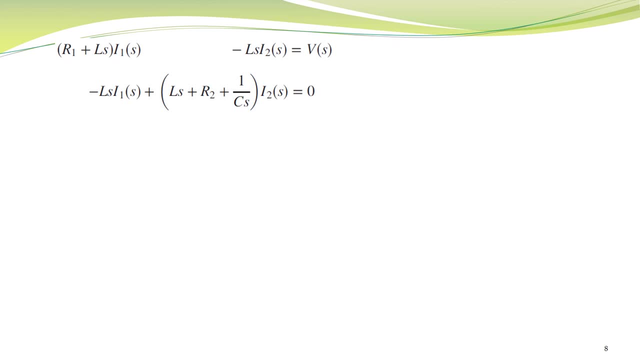 in current I2 and we take it as the output variable. To find the transfer function of the network, with V of t as input and I2 as output, we can use either elimination method or Cramer's rule. Applying Cramer's rule, we have I2 of S is equal to the determinant of this matrix. 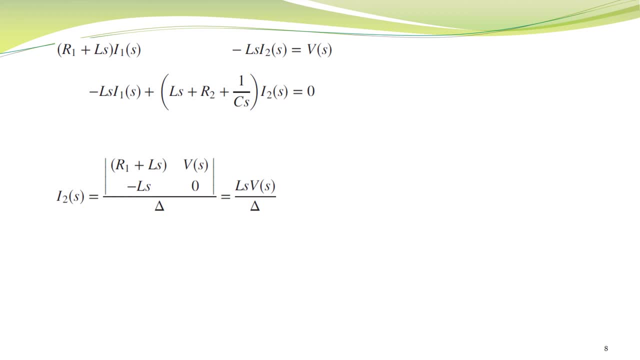 R1 plus L of S and V of S minus L, S zero, divided by delta, where delta is given by this determinant. So, after rearranging the T, the, after rewriting of, after expanding the determinant, we have this expression, That is, I2 of S divided by V of S is equal to LC S squared divided. 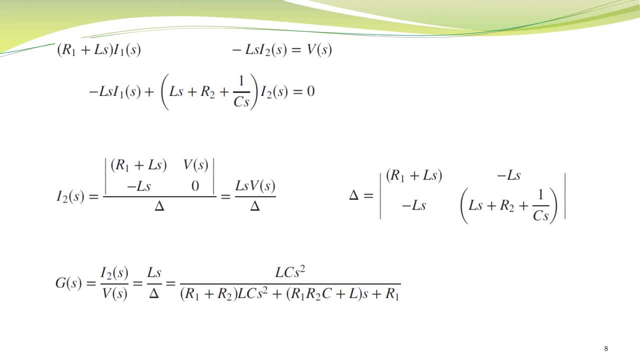 by R1 plus R2 multiplied by LC S squared. You can see that our range is very simple And therefore we will use the same expression, for example, the Zeta function. We can use this, we will use this, this reflection, and we will also use this expression for.